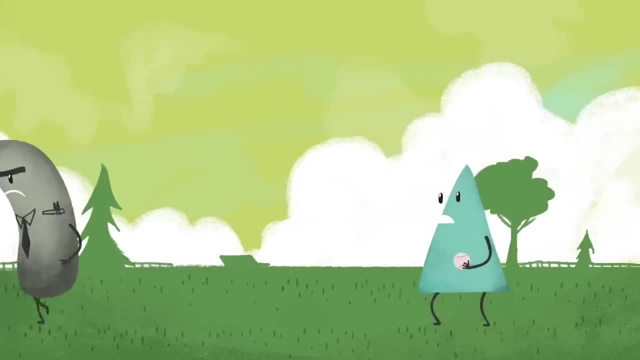 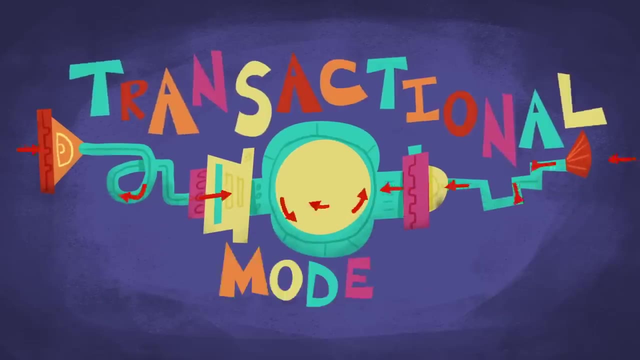 similar to someone tossing a ball and walking away. But in reality, this simplistic model doesn't account for communication's complexity. Enter the transactional model, which acknowledges the many added challenges of communicating With this model. it's more accurate to think of communication. 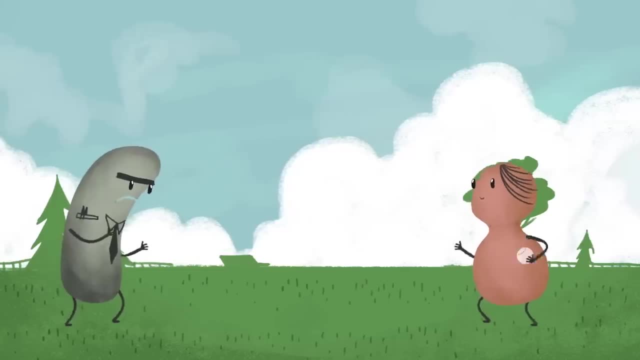 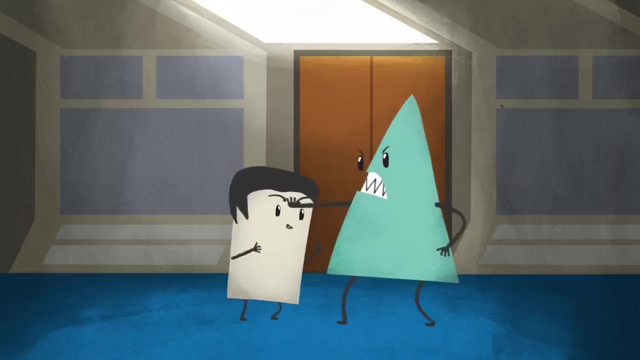 between people as a game of catch. As we communicate our message, we receive feedback from the other party. Through the transaction, we create meaning together, But from this exchange further complications arise. It's not like the Star Trek universe, where some characters can Vulcan mind-meld. 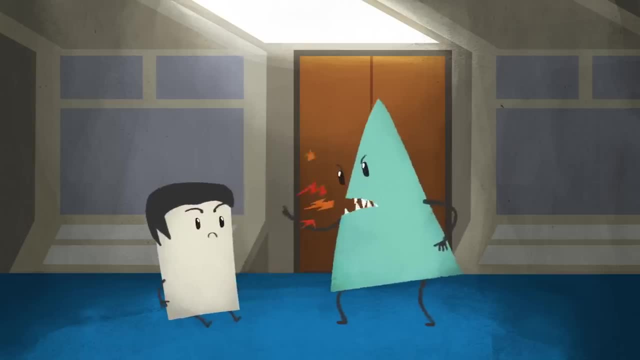 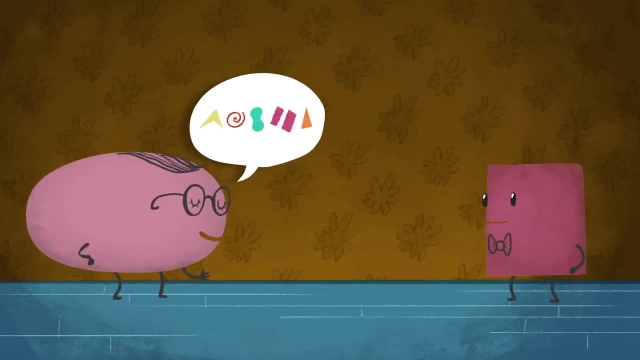 fully sharing thoughts and feelings. As humans, we can't help but send and receive messages through our own subjective lenses. When communicating, one person expresses her interpretation of a message and the person she's communicating with hears his own interpretation of that message. 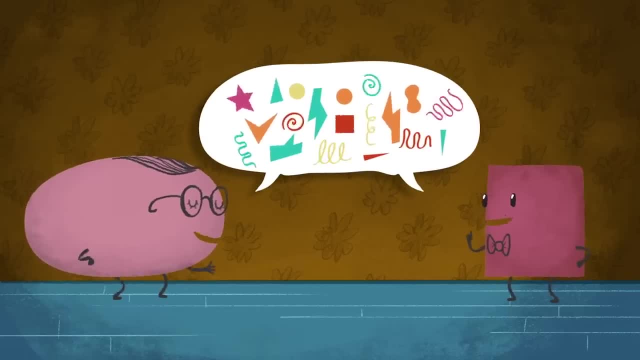 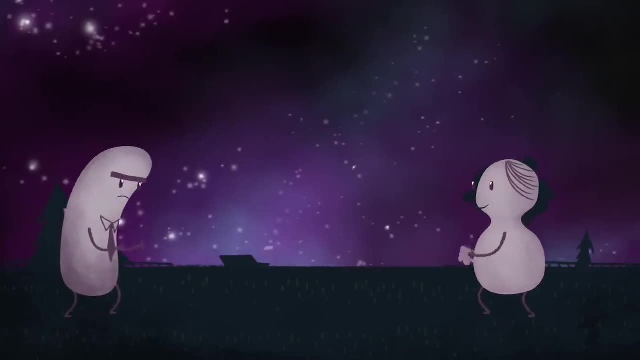 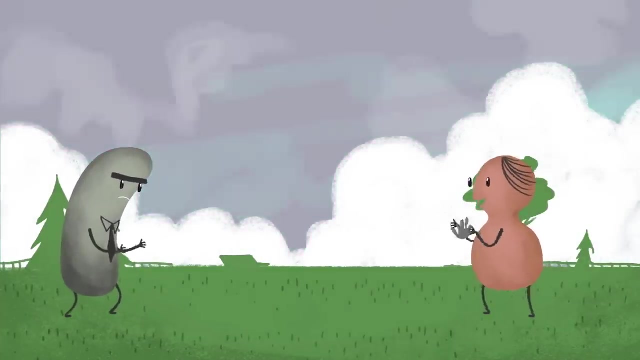 Our perceptual filters continually shift meanings and interpretations. Remember that game of catch. Imagine it with a lump of clay. As each person touches it, they shape it to fit their own unique perceptions, based on any number of variables like knowledge or past experience. 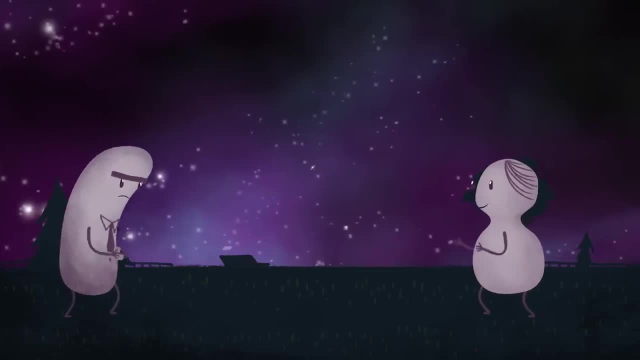 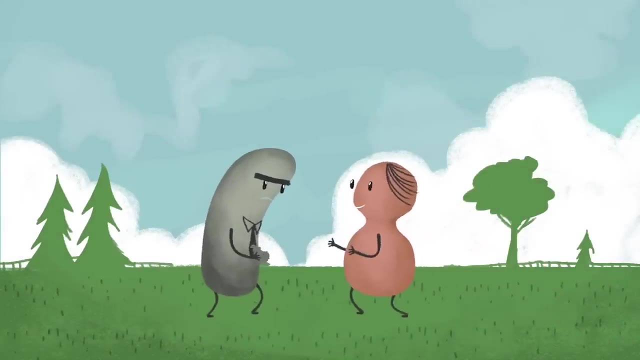 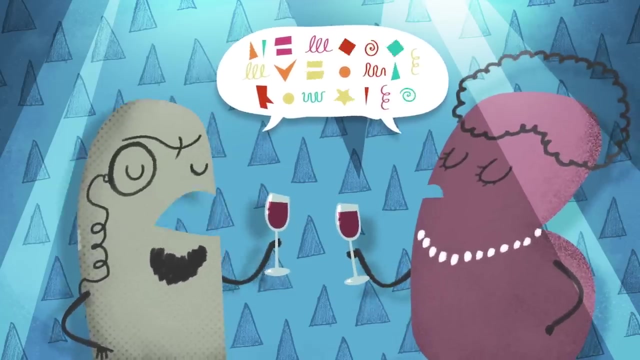 age, race, gender, ethnicity, religion or family background. Simultaneously, every person interprets the message they receive, based on their relationship with the other person and their unique understanding of the semantics and connotations of the exact words being used. 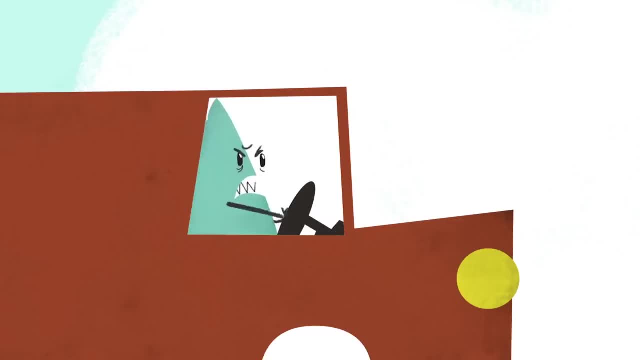 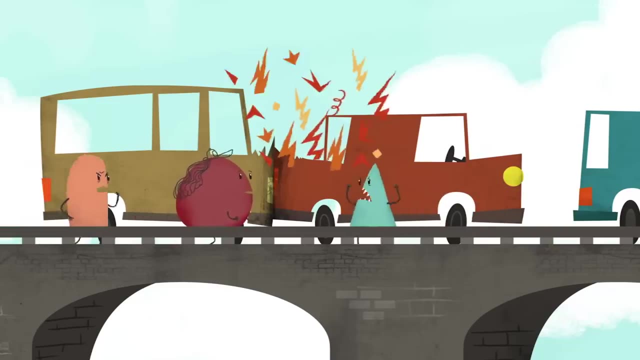 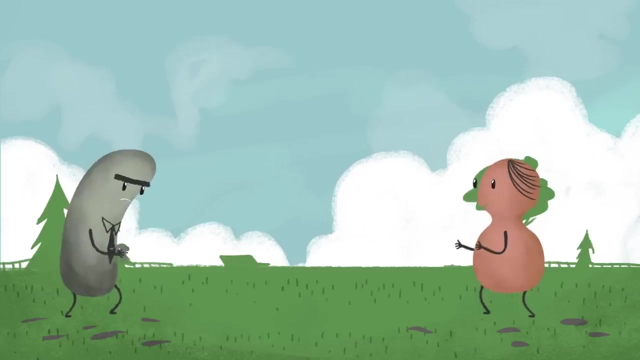 They could also be distracted by other stimuli, such as traffic or a growling stomach. Even emotion might cloud their understanding. And by adding more people into a conversation, each with their own subjectivities, the complexity of communication grows exponentially. So as the lump of clay goes back and forth from one person to another. 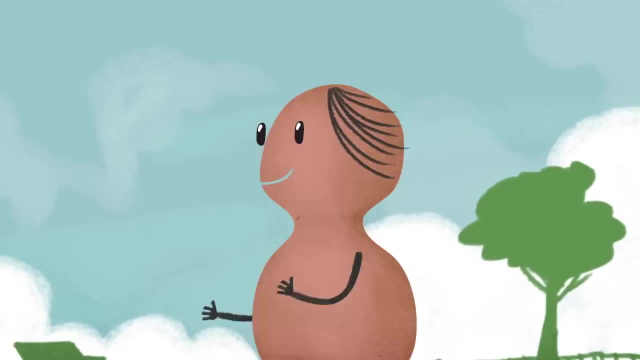 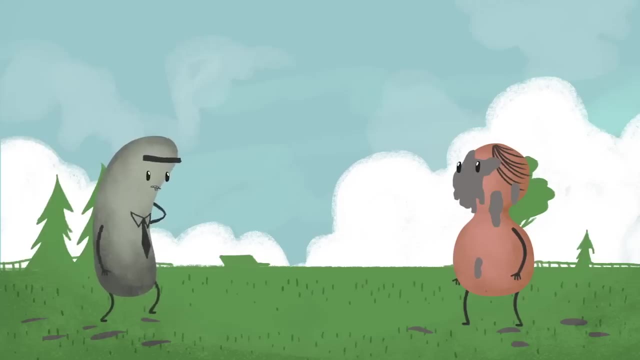 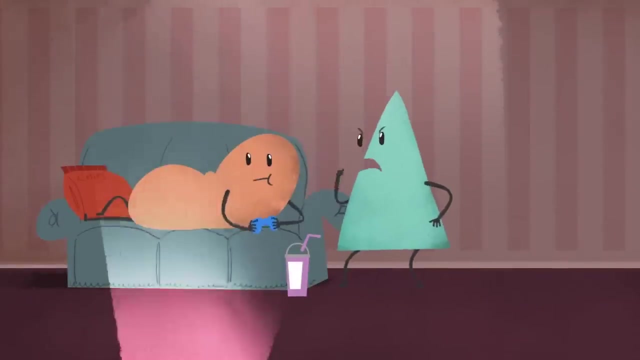 reworked, reshaped and always changing. it's no wonder our messages sometimes turn into a mush of miscommunication. But luckily there are some simple practices that can help us all navigate our daily interactions for better communication. 1. Recognize that passive hearing and active listening are not the same. 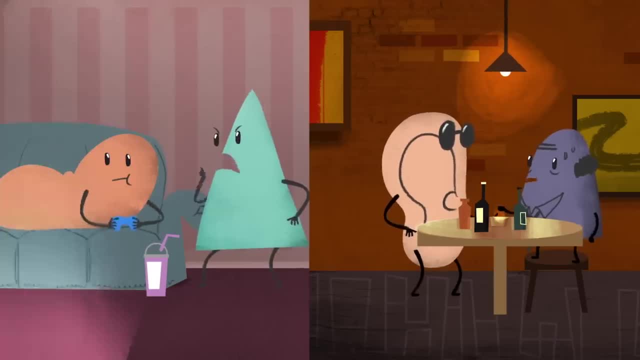 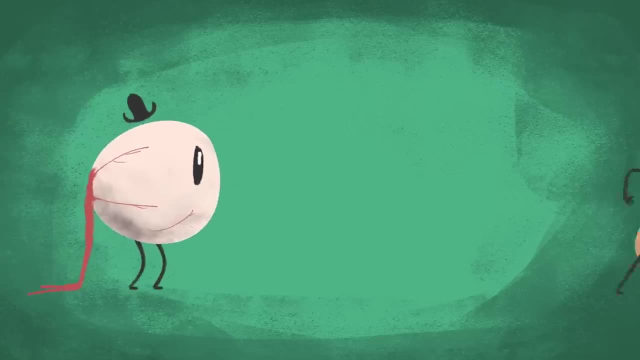 Engage actively with the verbal and non-verbal feedback of others and use them to improve your communication skills And adjust your message to facilitate greater understanding. 2. Listen with your eyes and ears as well as with your gut. Remember that communication is more than just words.